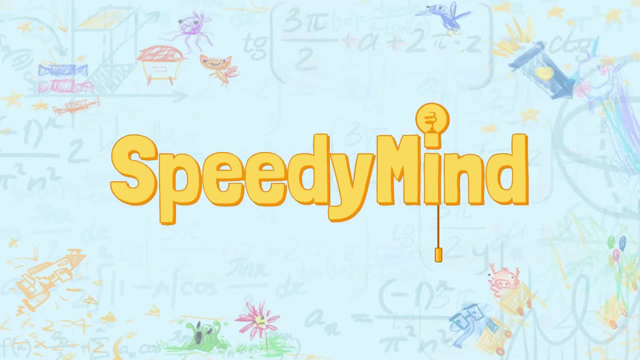 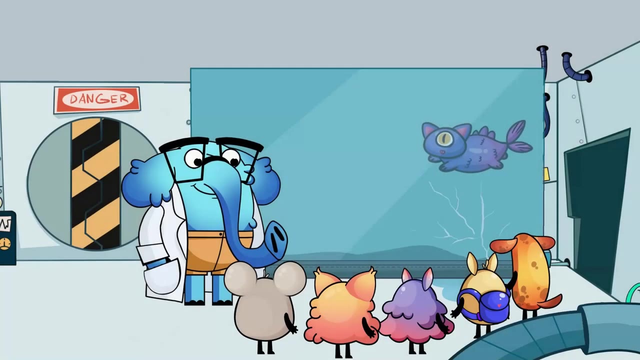 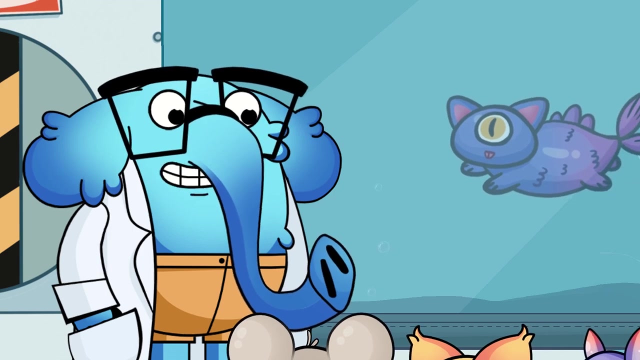 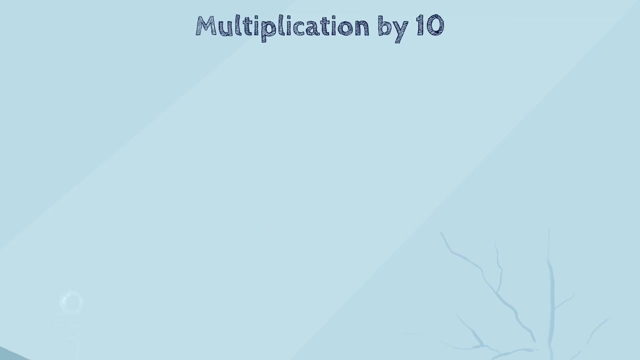 Hello kids, Good morning professor. Today we'll learn some tricks using multiplication by 10 and 5.. Let's start with multiplication by 10 and look at some examples. We know that 1 times 10 is 10.. 2 times 10 is 20.. 3 times 10 is 30.. 4 times 10 is 40. And 5 times 10 is 50.. Have you? 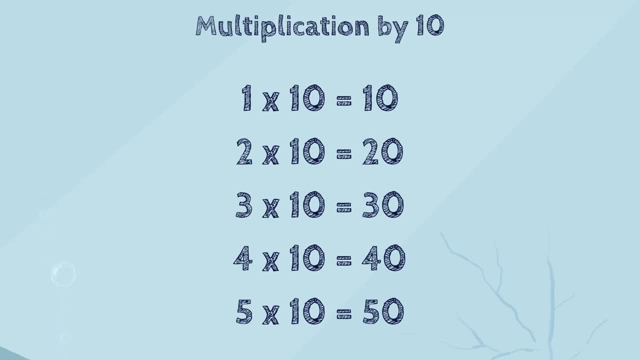 noticed something interesting, kids. It looks like you just add a 0 to the number that you multiply by 10.. Yes, absolutely. You've found the trick And I can say that it works for any number that you multiply by 10.. You just need to add 0 to it. So let's try 20 times 10.. What do you think? the 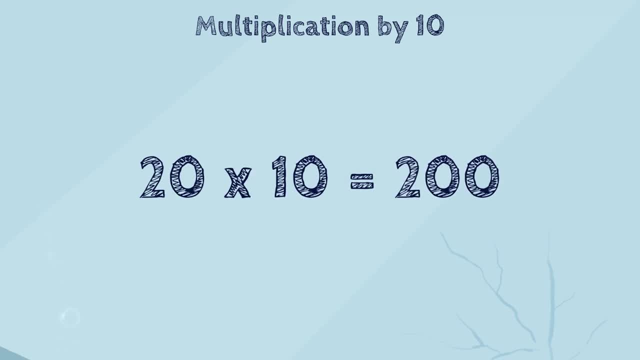 answer is 200!. Yes, and we all also know that the order of the numbers doesn't matter in multiplication, So this trick can still be used if 10 is the first number too. 10 times 20 equals 200, and 20 times 10 equals 200.. Let's try to solve another problem: What is 10 times 12?? 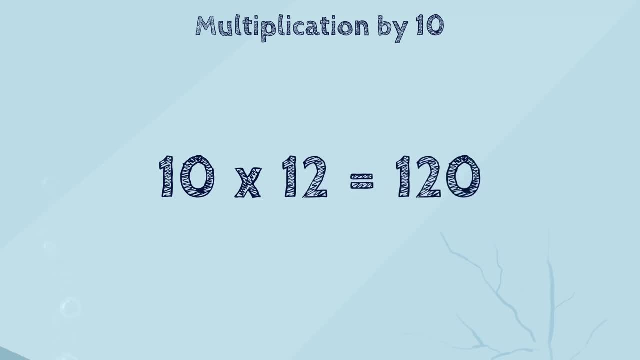 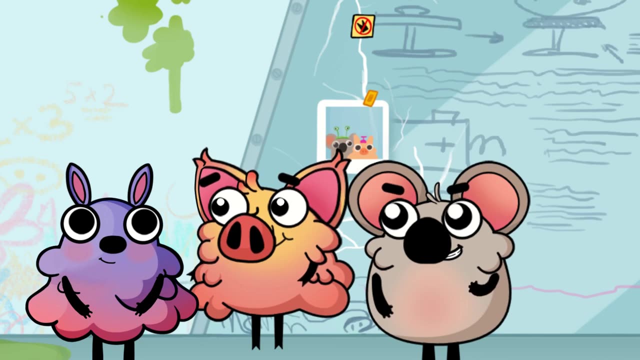 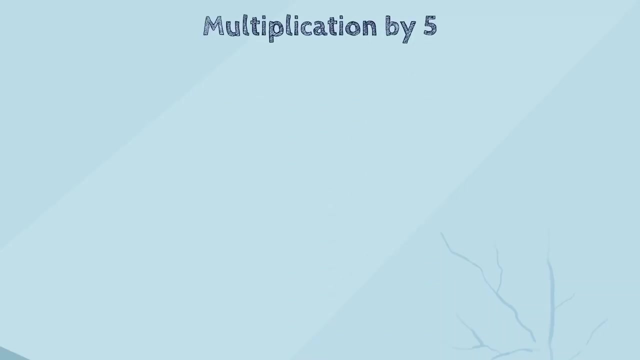 120!. Yes, that's it. I think you understand the trick. Yes, this is really helpful. Okay, now let's look at multiplication by 5.. What is 6 times 5?? It means that we need to add 6, 5 times, but we've just learned the trick to multiplication by 10, so you 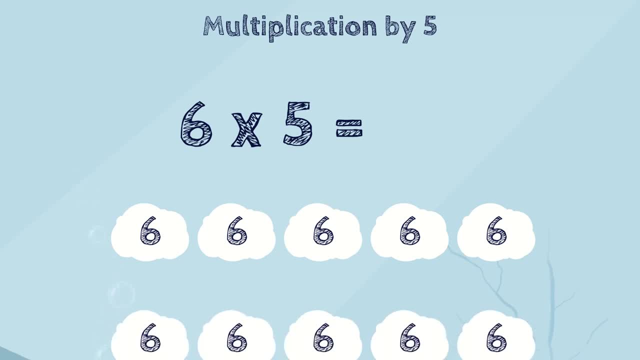 can easily find the answer to adding 6 10 times. You know that 60. Now what is 5 in comparison to 10?? Is 5 half of 10?? Yes, you got that. 5 is half of 10.. So to multiply any number by 5,.